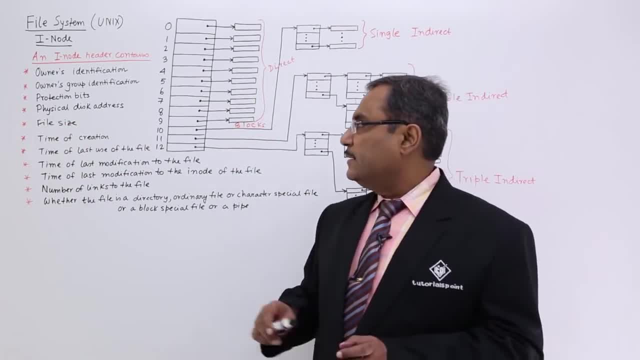 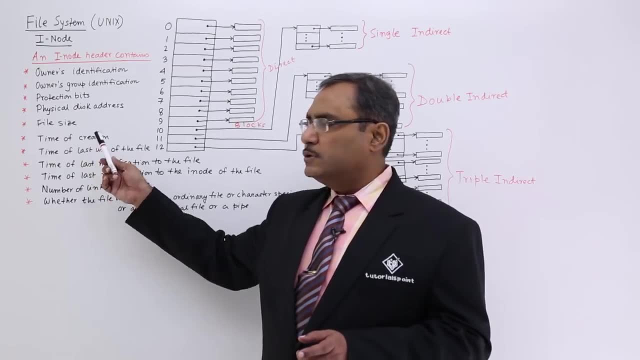 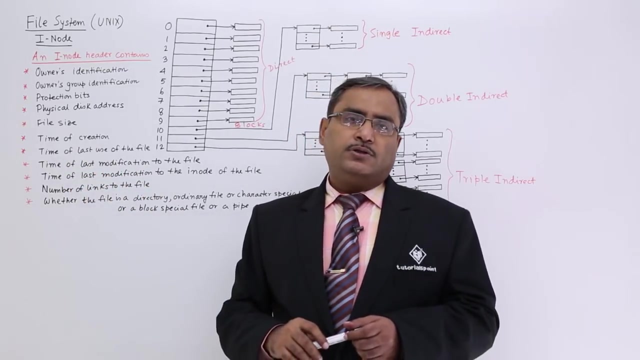 disk address to access the content of the file system. The file size, that is the total file size. Time of creation: to the from very word, it is quite common that it will hold the date and time of creation. Time of last use of the file. so what is the last time and date when this file has been? 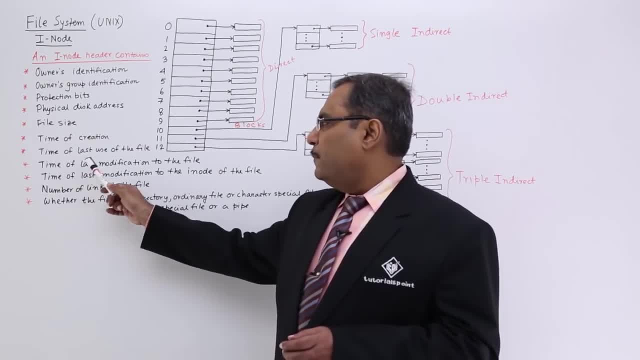 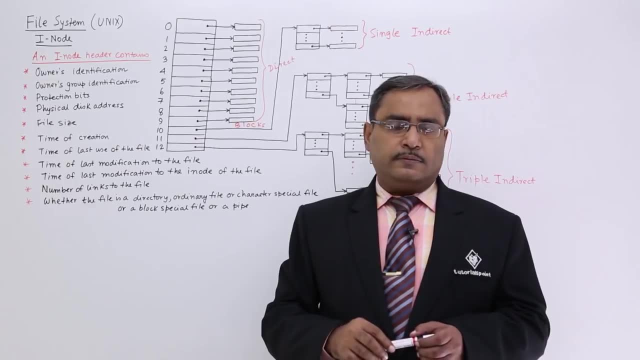 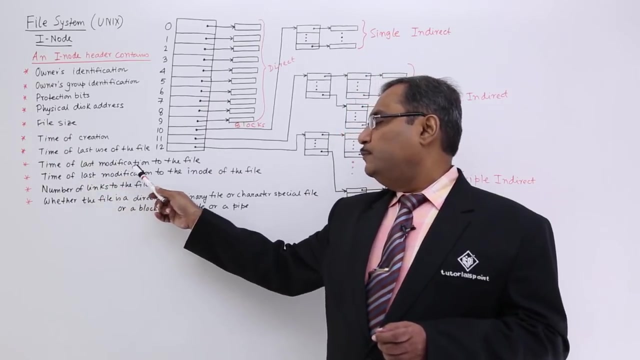 used, that will be kept in the header Time of last modification to the file. that means if you have changed some content of the file then the last time for the modification of the file will be kept in the inode header, The last modification to the inode of the file. so here the last modification to the 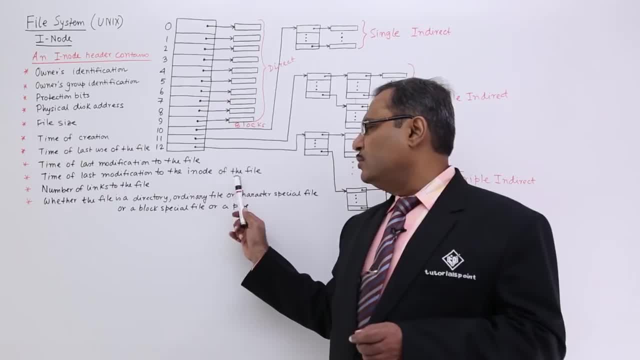 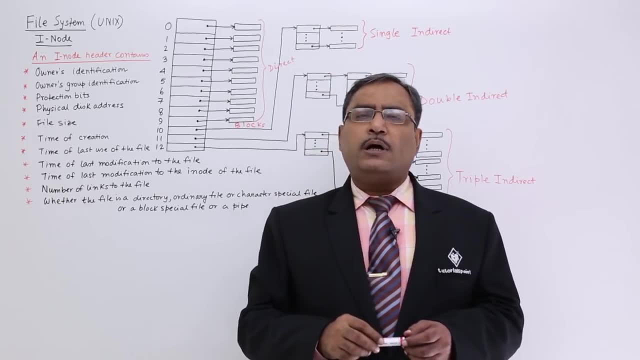 content of the file. Here the last modification to the inode of the file and the respective time will be kept in the inode. What is the? what is the meaning of this modification to the inode? Let us suppose I am going to change the protection bits. 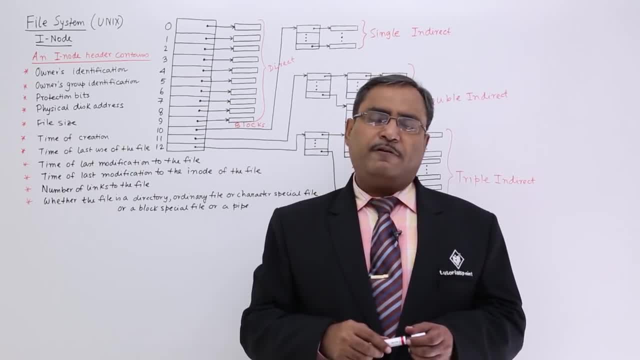 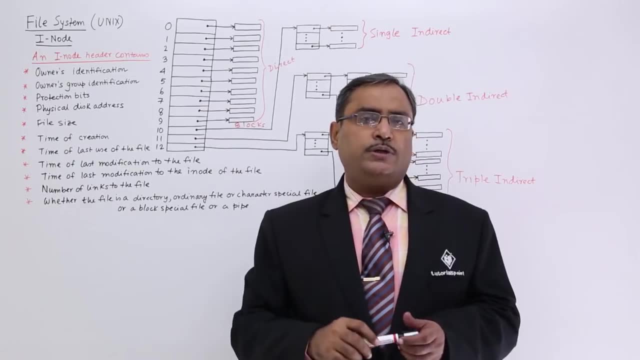 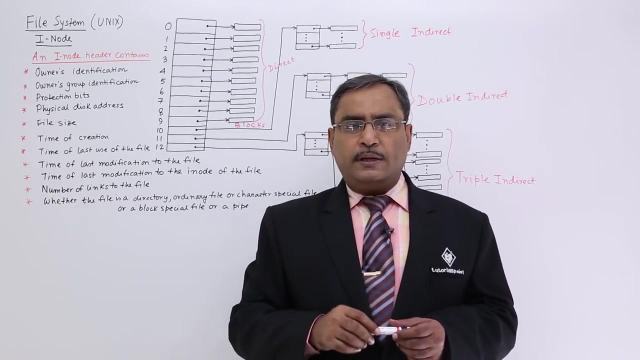 Let us suppose I am going to change the user ownership of that particular file system, user identification number. Then obviously the file content is not getting changed but the inode is getting changed. Number of links to the file. In our laptops, in our desktops, we used to have some shortcuts on our desktop. 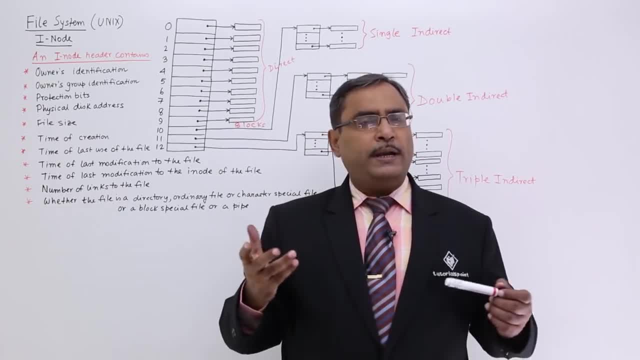 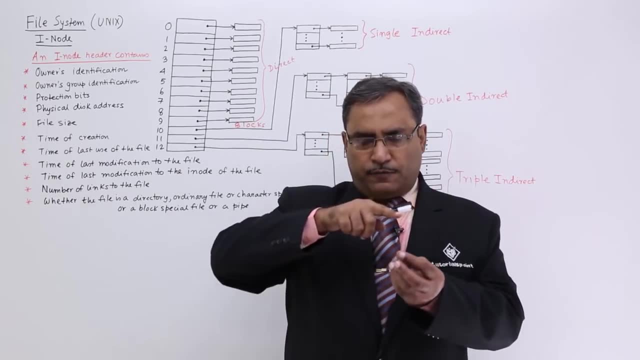 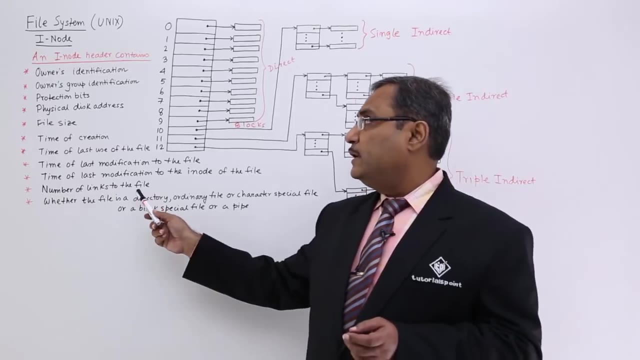 If you click on the shortcut, then the respective application will get open and can get run. In case of Unix operating system also, a file can have different links from different paths, so that the file can be accessed through those paths and number of links will be kept in. 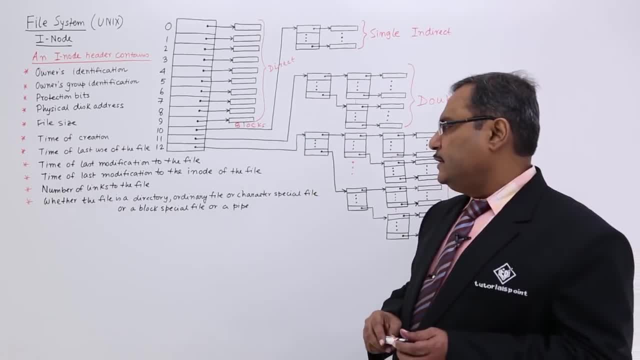 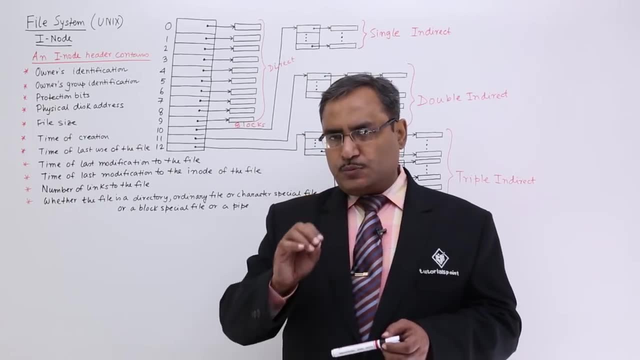 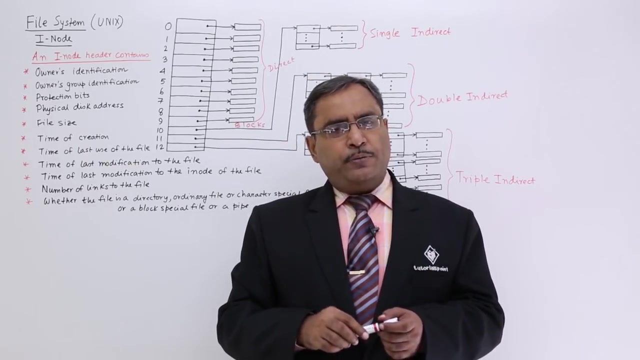 the inode header. Whether the file is a directory, ordinary file or character special file or a block special file or a pipe, that identification, that corresponding indication, will be kept in the inode header. A file can be ordinary file. that means a character file. In case of Unix operating system, all the I O devices will be mapped. rather, I should use 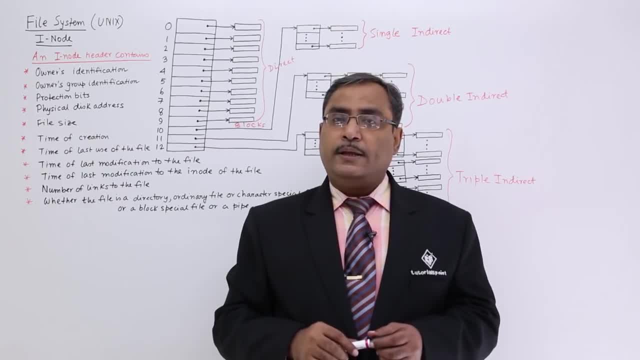 the technical term- will be mounted on a file system. All the I O devices can be categorized into two heads. One is a block special file and another one is a character special file. Mouse and printers are the good example of character special peripheral device. 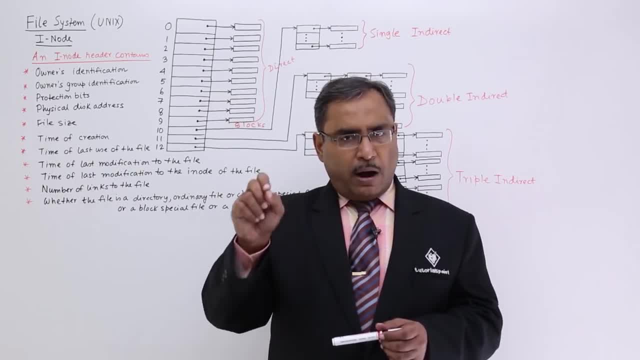 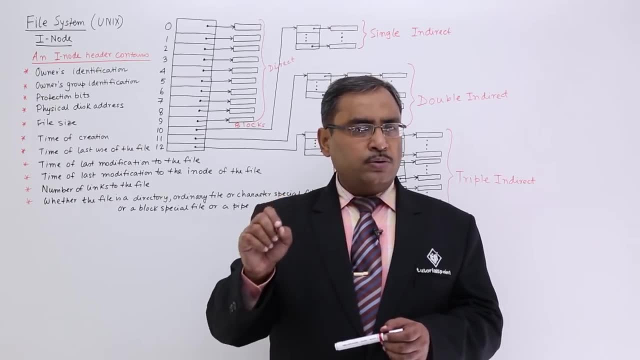 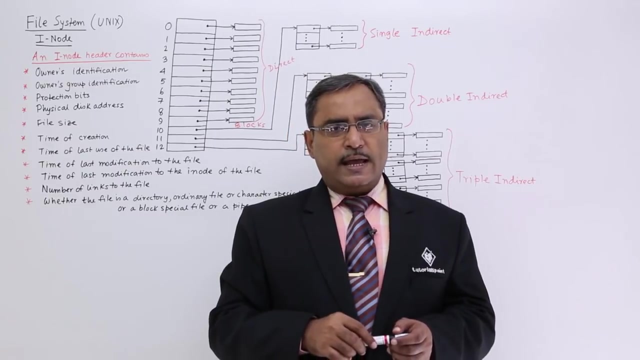 If you, if you just move one mouse or if you click a mouse, then mouse will return one byte of information, or streams of bytes of information, to the computer. That is why mouse is communicable through bytes, characters In case of a hard disk. in case of hard disk, can I read a single byte? no, I am supposed. 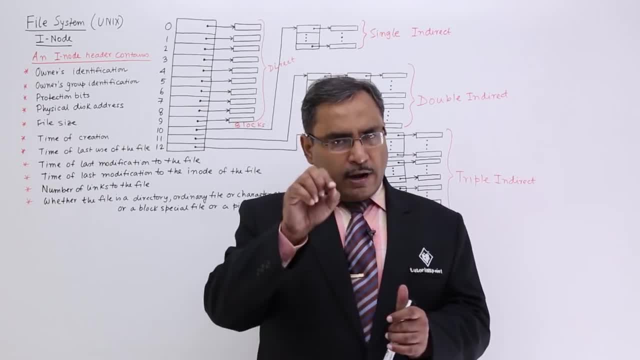 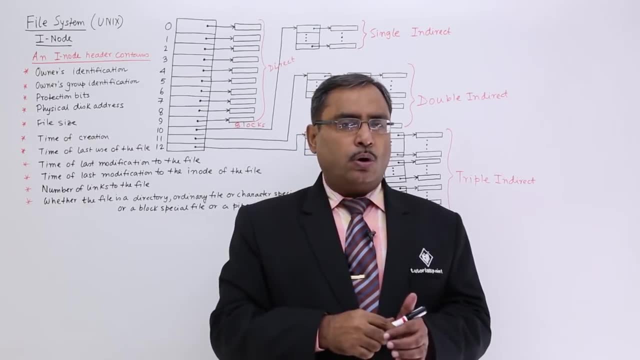 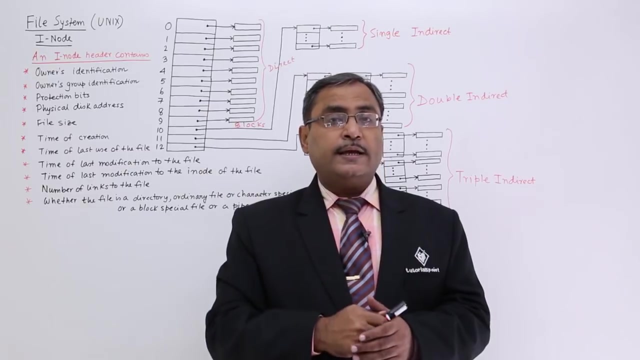 to read a block known as the allocation unit. Can I write? can I put a single byte in the hard disk so that only the bytes amount of space will be reserved? no, it will occupy a chunk of bytes for the operation. So that is why your disk is a block. peripheral device. 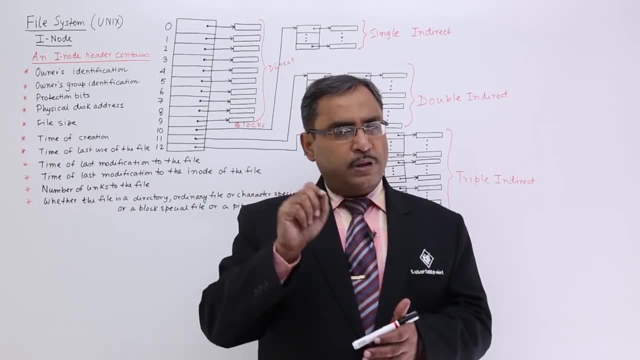 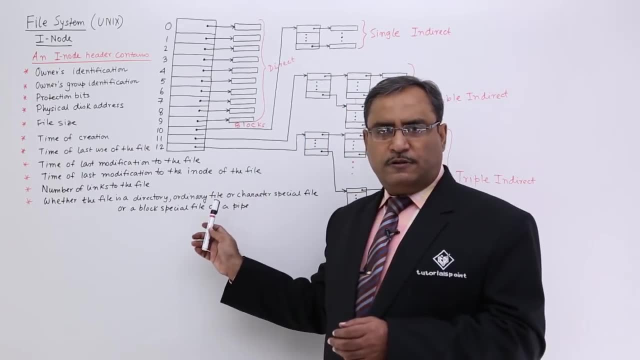 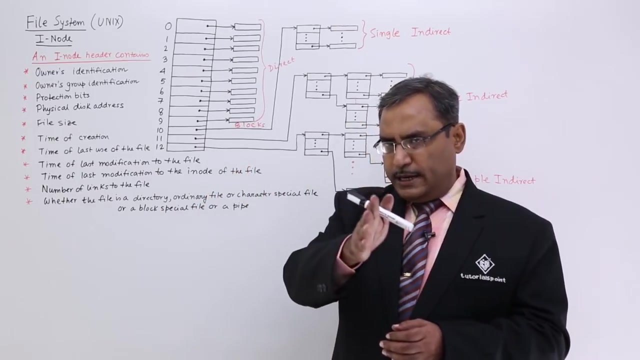 Can I print a single letter A on a piece of paper through a printer? Yes, you can do, because printer is a character special file. So, depending upon the character special file or block special file, In case of Unix operating system, the corresponding device will be interfaced through a file system. 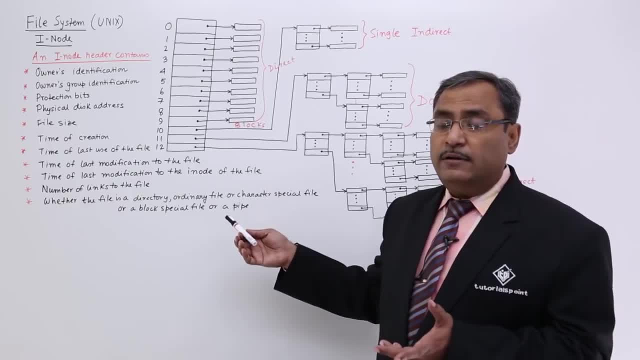 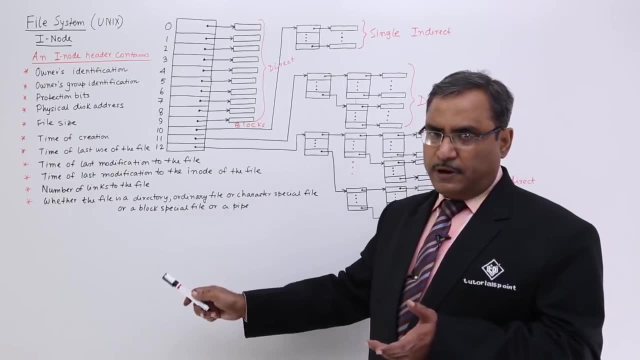 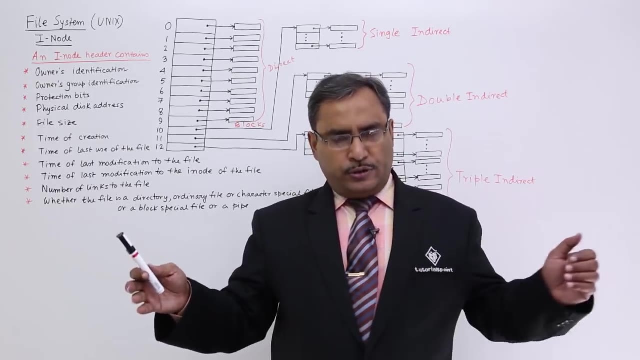 in the Unix operating system. So what is the nature of the file for which this I node is there? Is it an ordinary file or a directory, or character of block, special file or a pipe? Pipe is nothing but a file which will take some inputs and which will produce some outputs. 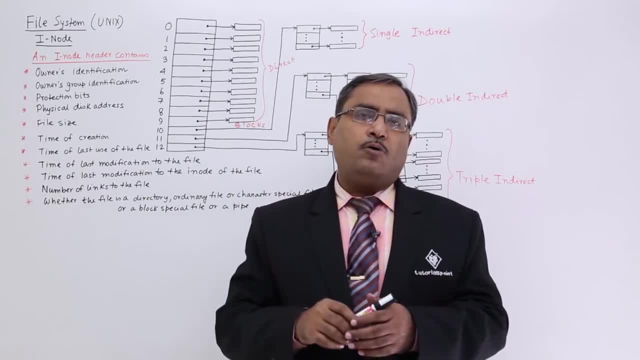 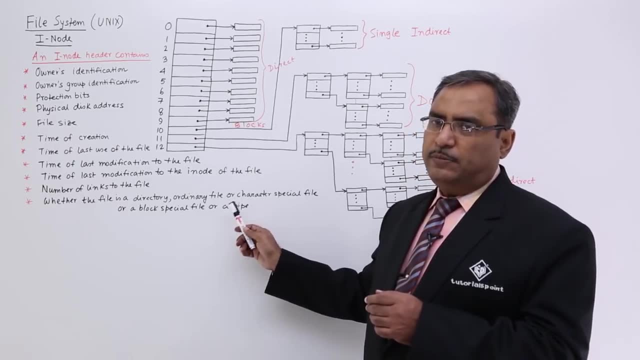 So it will take some inputs and then it will redirect it to the output. So there, the pipes are there pipes are the files. some pipe files are there, So it will indicate whether what is the type of the file to which it is pointing. I node is having a data structure like this. 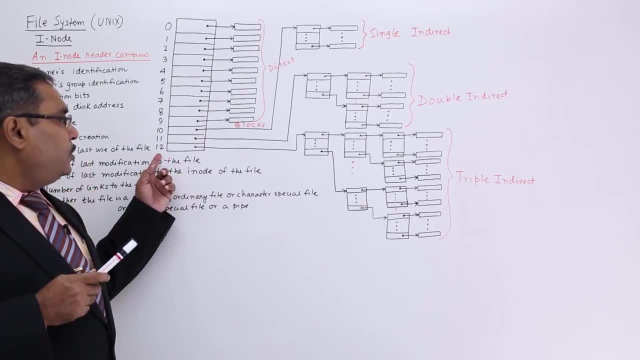 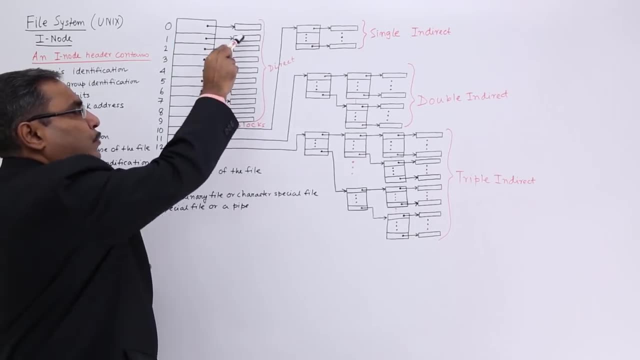 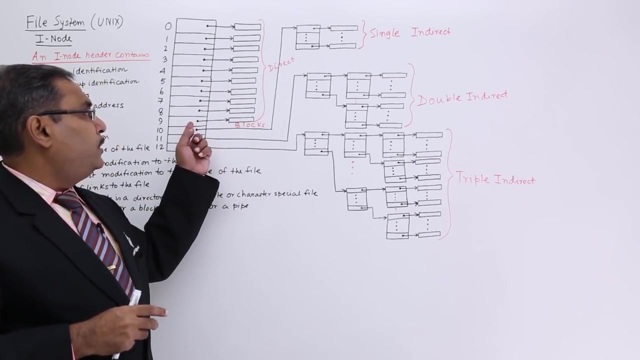 It is having 13 fields, as a field number is starting from 0, so I am having a 12.. So it is having 13 fields. first, 10 fields- 0 to 9- will have the direct block address. So these are the blocks which will be containing data, that is, the files content and this particular. 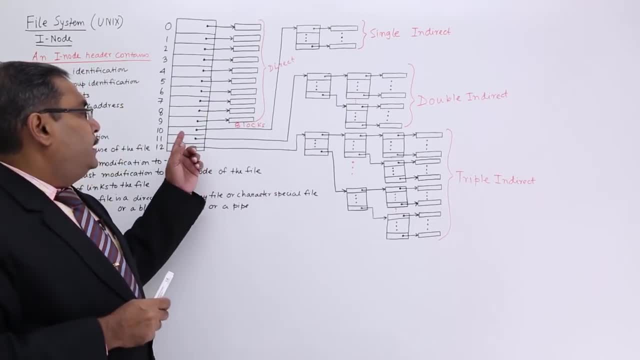 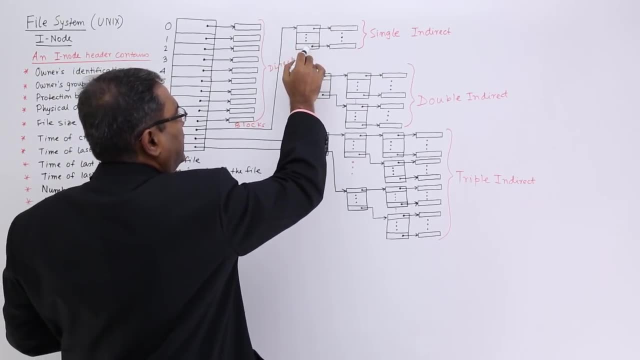 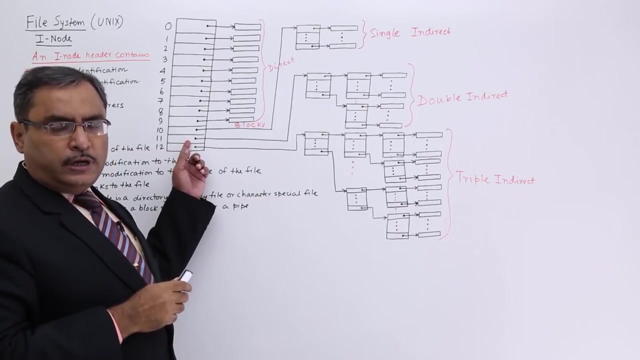 pointers will be pointing To those blocks. the 11 field will be containing the indirect block address. that means it will be pointing to a block which is nothing but index, and they will be pointing to the respective physical blocks. And the 12 field will be containing thus double indirect. that means it will be pointing to